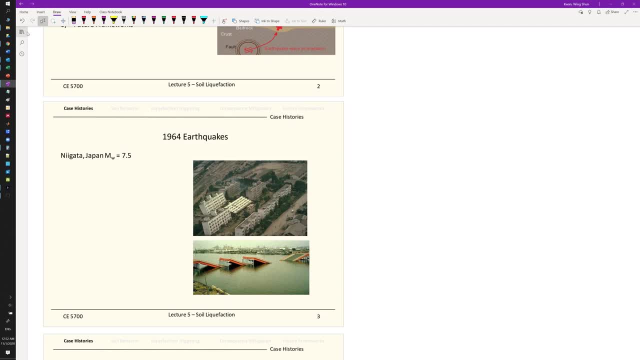 it has been happening in human history for a long time. it has been happening in human history for a long time, Back to some old days. documentations maybe like a couple of hundred years ago. some even date back to almost like a thousand years ago. 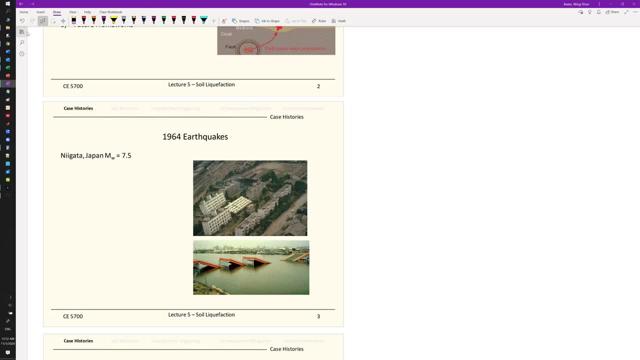 in some transcript maybe from Japanese or some other very old developed countries. in some transcript maybe from Japanese or some other very old developed countries. But what started for the engineering communities is starting on the events of the. But what started for the engineering communities is starting on the events of the. 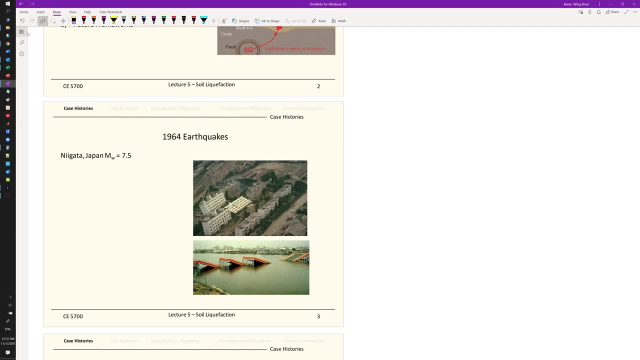 back-to-back earthquake in 1964.. So there's two major earthquakes happened in 1964.. First is the Niigata soil aquifer fractions earthquake. This happened in Japan. So the classic picture here is, you know, is also the cover picture of your Kramer textbook. 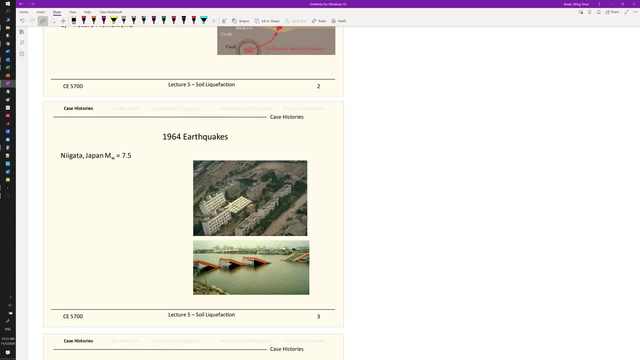 So what happens is this famous cave history at Niigata. So what happens? is this famous cave history at Niigata, the? you see some apartment building right there. What happened is those building is designed as shallow ground, shallow foundations And the footing- the main footing- is sitting on liquefiable sand layers. 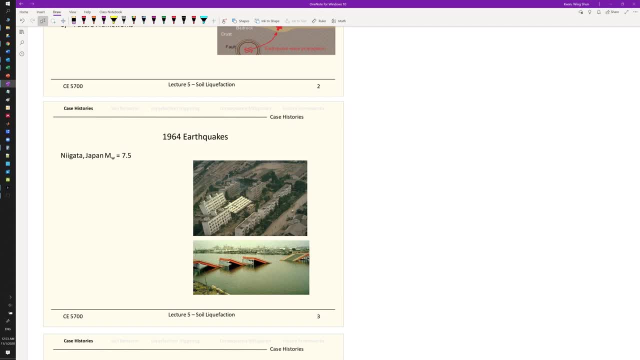 So back to the time more than 50 years ago. at that time, the civil engineering communities still don't have a good understanding of the building. at that time, the civil engineering communities still don't have a good understanding of the building. the building code adjusts the soil aquifer fraction issue. 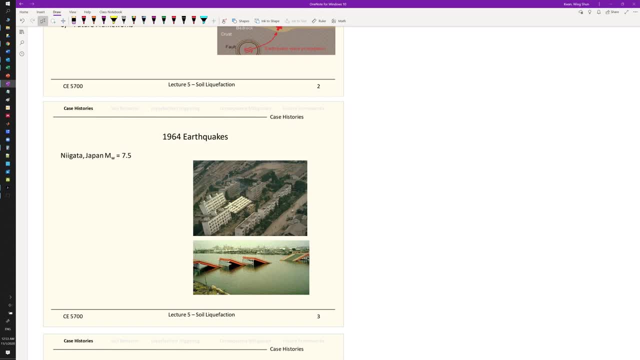 So back in the old days. you know, people don't check for soil aquifer fractions. So the shallow ground foundations pretty much is sitting on liquefiable soil layers. So when earthquake happens you liquefy the soil, then you have tipping effect: the building just tip over. 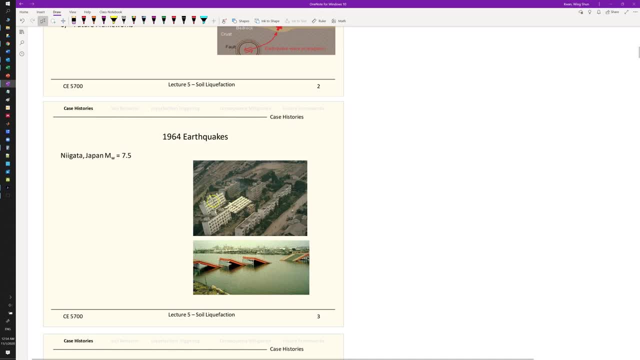 And you see that it's not like a structural problem. And you see that it's not like a structural problem. And you see that it's not like a structural problem. The structure is fine, you know, just like a box tip over. 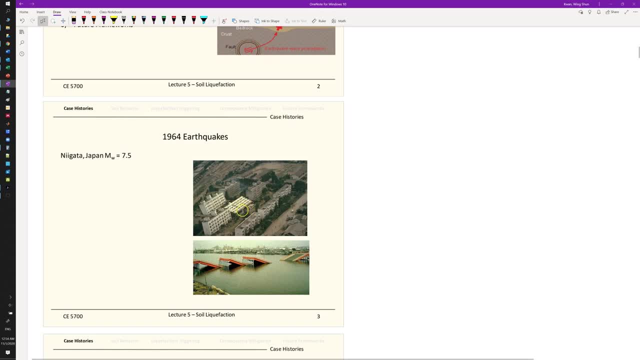 Since what happens is at the shallow ground, the main foundations, it just cannot support the building anymore. right, It's all got liquefied. So that's a very famous cave history of soil aquifer fractions. So after that, after 1964, you know, it may take another five to ten years. 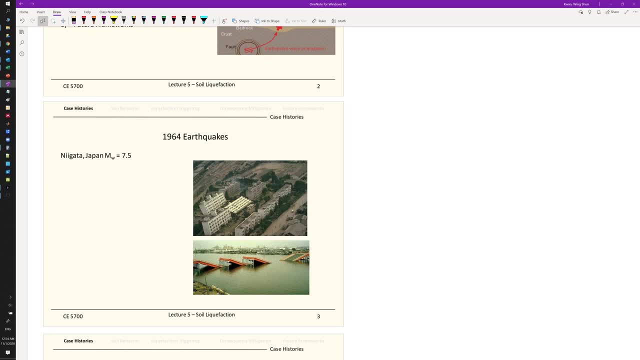 three to ten years for research and then for results coming in to building code. three to ten years for research and then for results coming in to building code is no longer allowed you to build a build a of a matt foundation on liquefiable sand layers anymore. 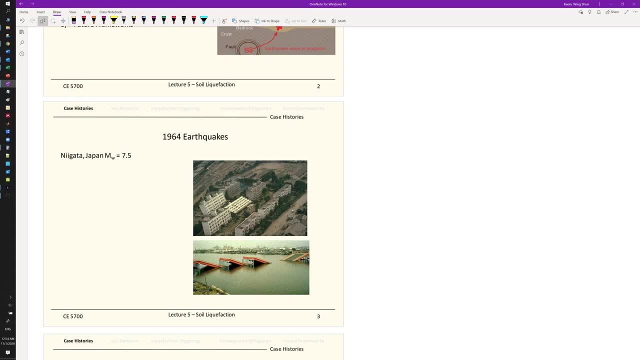 For example, if you in California, if you have again, if you have kind of like similar apartment buildings, if you find like saturated, you know, as an example, if you find like a saturated, you know esca climate even though you know. it's not a natural при Herrenya situation. It's good, It's better. It makes more sense to be 2500 and so on. It's good, It's good. It's good, It makes more sense to be 500 and so on. 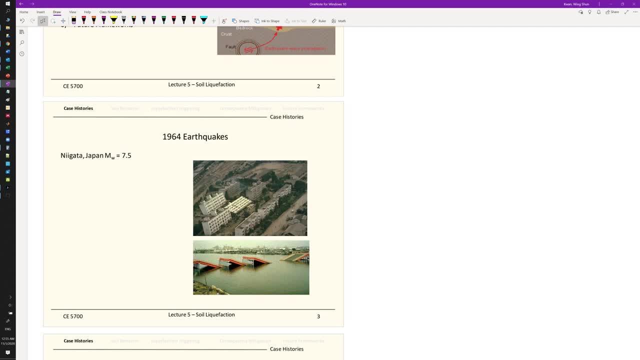 the potentials to be saturated, liquefied the sand layers. You cannot just build a shallow ground foundation on top of it. You have two choices: either you have a deeper foundation, bypass the liquefiable soil layers, or you need to do ground improvement, which means, like some, 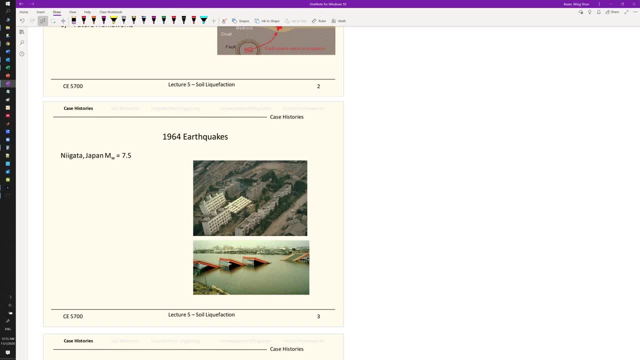 grounding. You need to densify the sand layers. you know that's a need to be get done now since the 1964 earthquake. and also you know a huge of a lot of like a literature and you know, get on documenting this. after a decades or two decades of research, people finding all this phenomena, 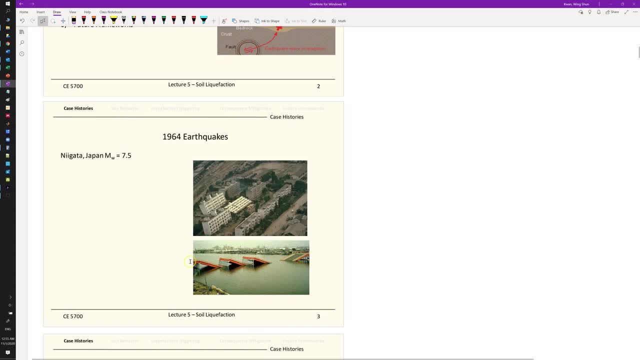 And the picture here in the bottom. so you're a bridge. and also soil liquefaction is. one of the consequences of it is lateral spalling. So when soil liquefaction happens, the ground can deform quite a bit of this displacement. So in this case it's kind of like 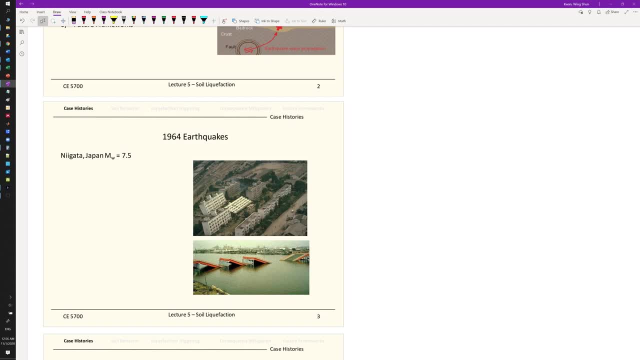 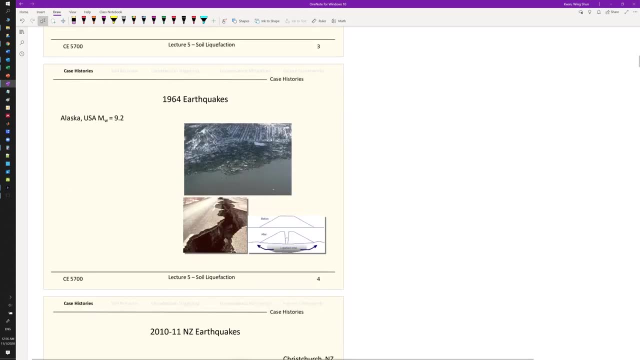 spread out the footings of the bridge. So after the earthquake events the bridge just collapsed. So at the same years, the great earthquakes- that has some earthquake magnitude of 9.2 also hitting Alaska. So that's the another earthquakes sequence happened in the same year. It also, like, caused a lot of slope problems. 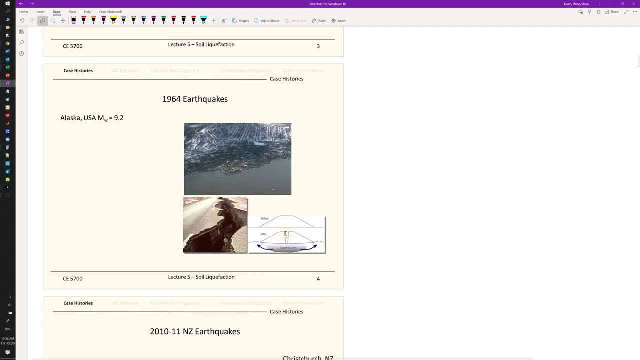 and it kind of like crack up a lot of embankment that happen that located in Alaska and you can see, like you know, highway there, when, when the ground deform, How you can tee up the, the earthwork, So it also features features a lot of landslides. 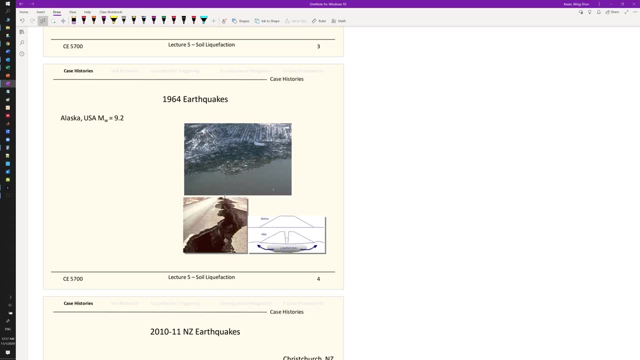 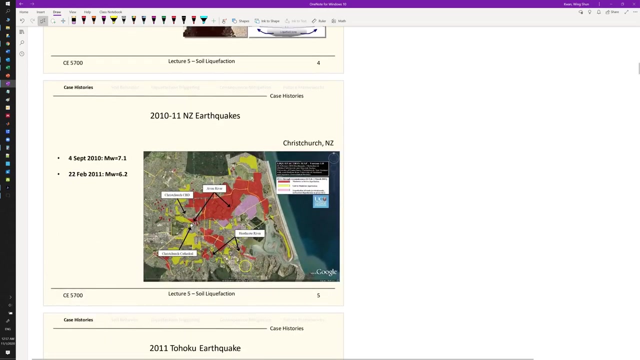 so earthquake can introduce a landslide, uh, when? uh, uh, you know, when the energy releases the ground. so, uh, 1964, uh is is kind of like an important year uh in the uh, the topic of solar refractions. so we turned the clock, uh, you know, just like a decade ago, uh, and also another important uh. 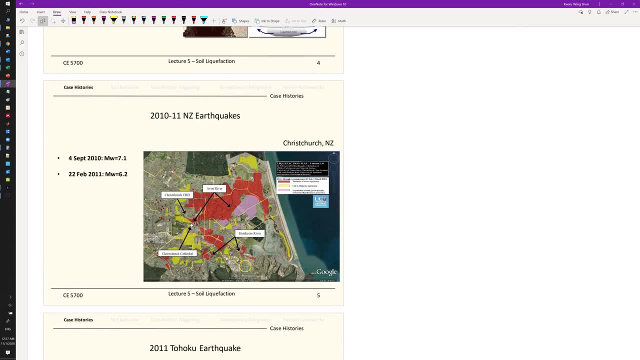 uh earthquakes uh k history that uh happened as christ church uh new zealand. so in between, like 1964 and uh 2010, there's a lot of like earthquake happens and also features with uh local factions. you know for sure the 1994 the north, which earthquake you know. you also have. 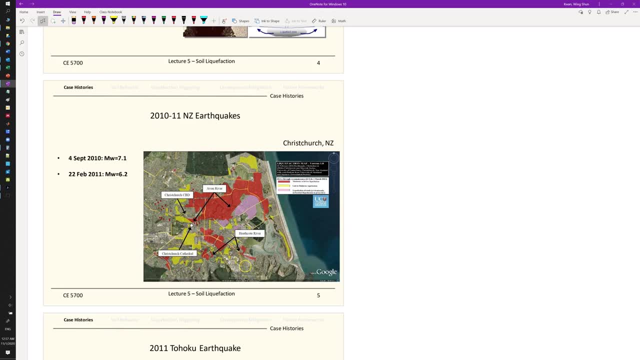 some liquid factions events going on. uh that uh happening in california: have southland california. you know you also have uh uh some liquid factions events going on. uh that uh having a california- have southland california. but another important worldwide is the 2010 uh new zealand earthquake. what being uh a special about? 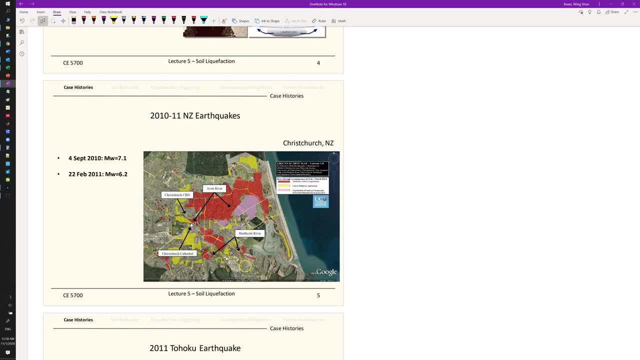 this earthquake is uh uh. we kind of learned something new. so every major earthquake, when it happens, you know it's always like a teachers teach us something, and but for particularly this one, it teaches: uh, in solar group fractions is uh uh. when the ground get electrified, uh, it can be. 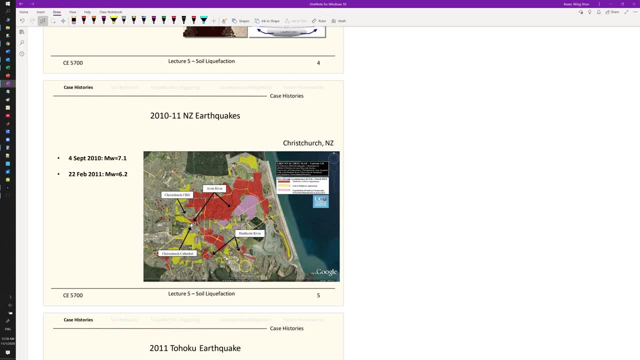 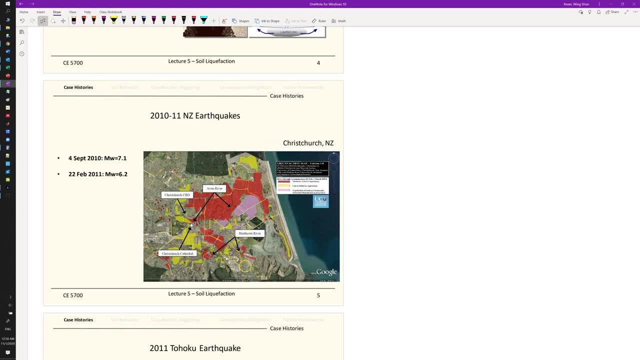 we have a general belief that, uh, when after liquefaction happens, it kind of like release the excess pore pressure and densify the ground, so you're, you know, you have you kind of like, you know, uh, making the sand with a higher density and then so, uh, you kind of prevent you to uh for this. 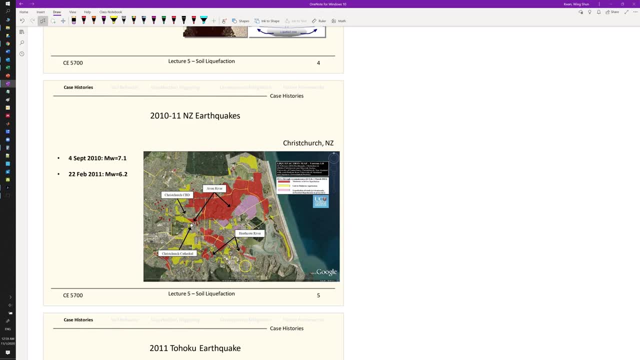 for the soil to be liquefied again in the near field, you know, near future. but this, uh k history just uh, give us another lecture. that indeed, uh, solar coefficients can be happens, uh again, uh, you know, after like, even like a full short or after short, uh, uh, the ground can be, uh can be. 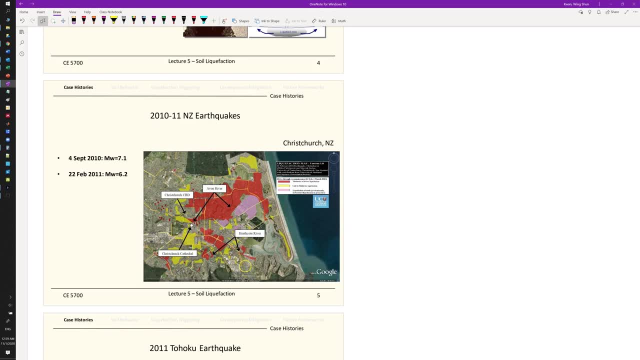 again uh, liquefied and uh, this happened and this uh k history happened after christ church. so the map here is: when you the downtown of christ church and it's, it's, it's a very uh, uh dangerous earthquake, as you can see uh in the graph, in the graph, in the picture there. so the red color there highlight uh, the uh. 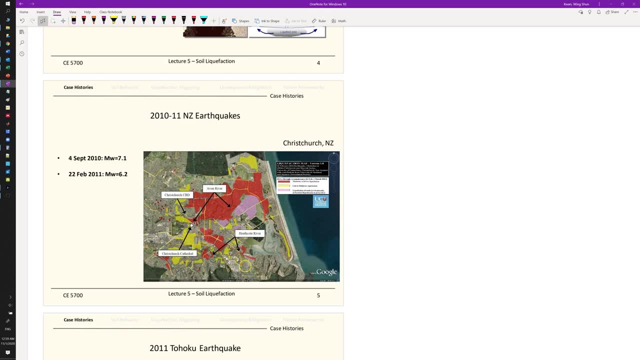 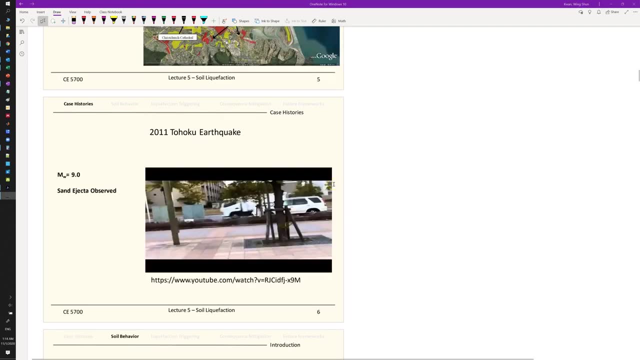 the area that uh. uh, he has a serious uh survey damage uh because of a solar. okay, next, uh, um, i'm putting social videos uh. that uh is from the 2011 uh tohoku uh earthquakes. um it. this is uh a uh quite like high quality video that captured uh the event of solar liquefactions. 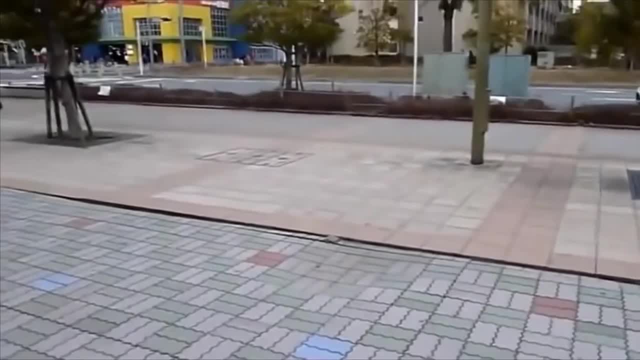 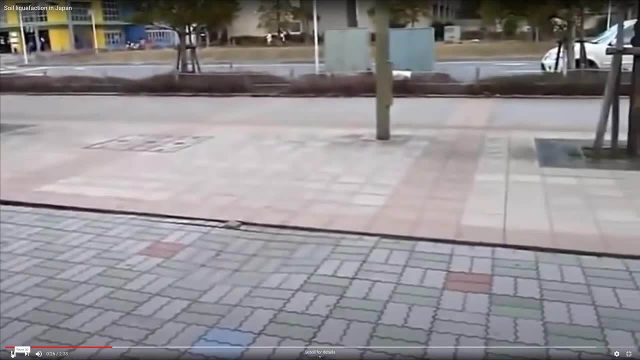 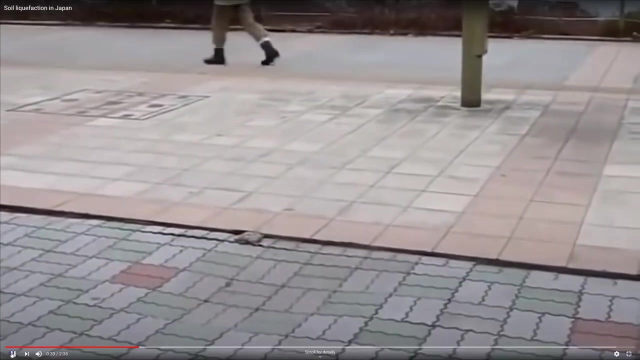 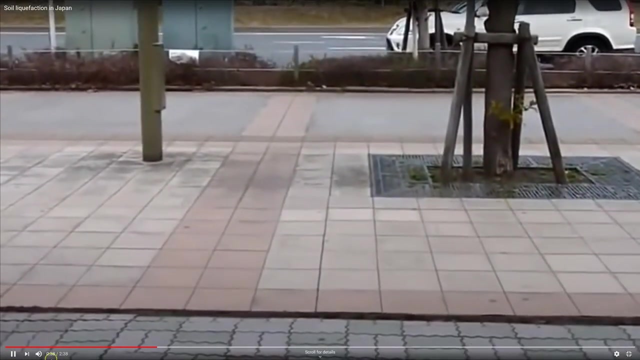 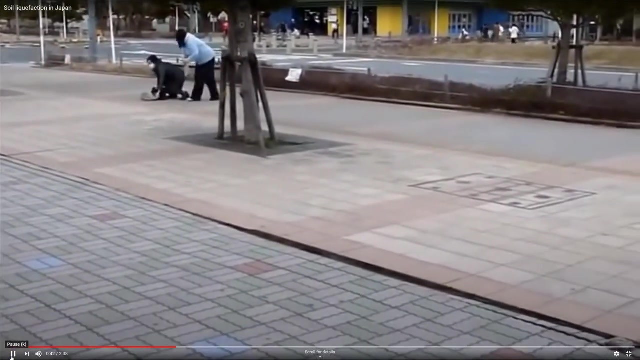 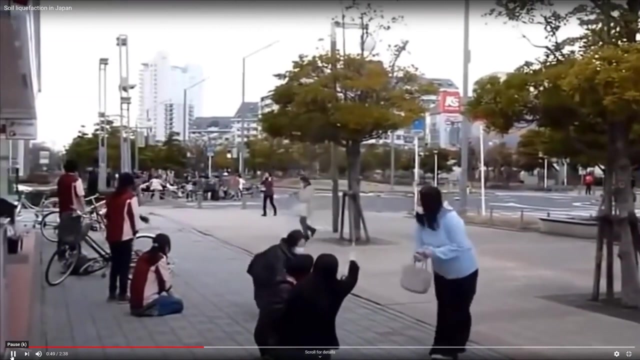 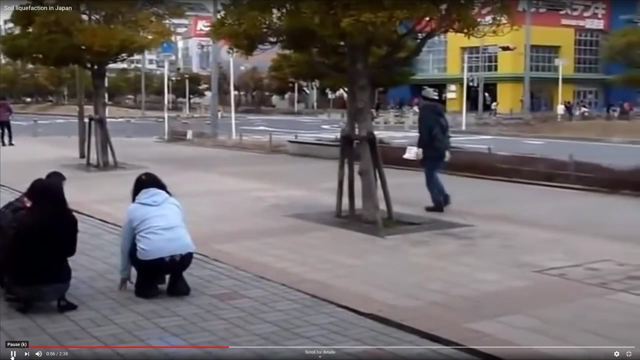 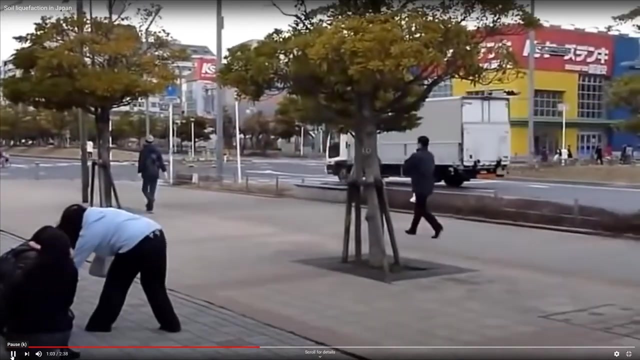 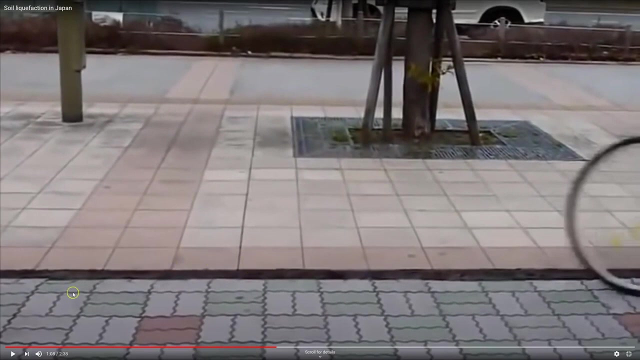 so you see the ground, uh, the ground start to shake. see all the lateral movement over there. you can see that over there they're easier to see. um, this is he's probably been having a swelling thing before. what was that? you see how they're growing like: um, they move, uh, you, these. 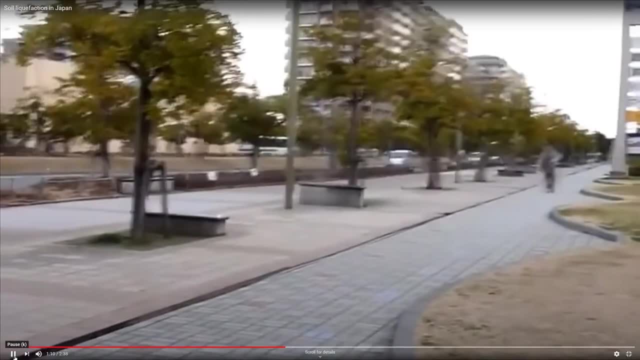 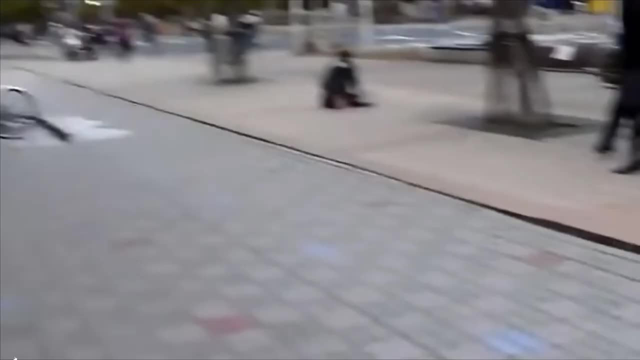 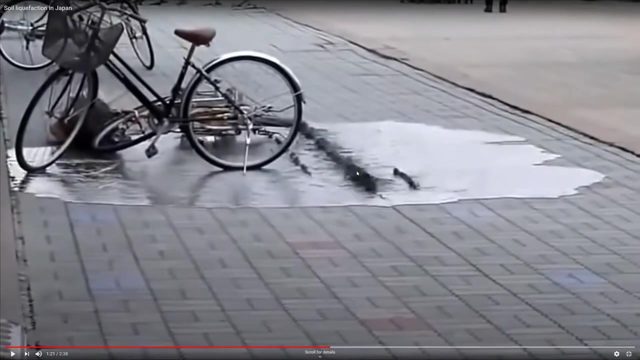 lotions and stuff like that. can you see, they've it, check it, they move right here. they're veryulla relatively each other. So here you start to see the evidence of solid liquefaction. So they call it either sand boils or each other. What happens is, when liquefaction happens, it generates the excess pore pressure. 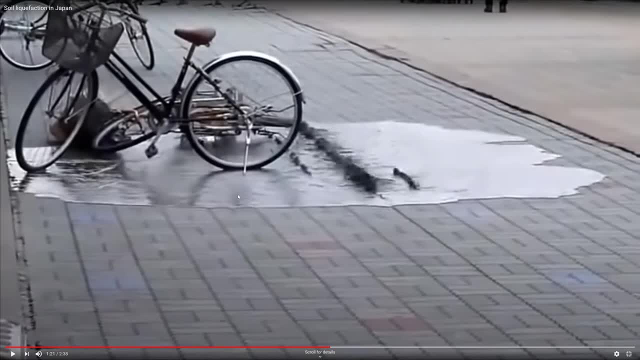 For the excess pore pressure to escape the ground or the sand layers, just like your consolidations that you learn in CE366.. So the excess pore water pressure either only can shoot up or grow to the next more permeable layers underneath it. But since you're working on sand, 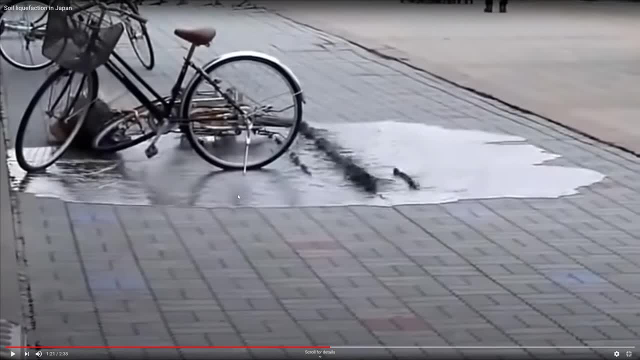 So it's very hard to find other layer of soils that is more permeable than sand layers. So, very likely, when solid liquefaction happens, the excess pore pressure will shoot up to the ground. So that is what engineers will try to confirm solid liquefaction happens if they see the 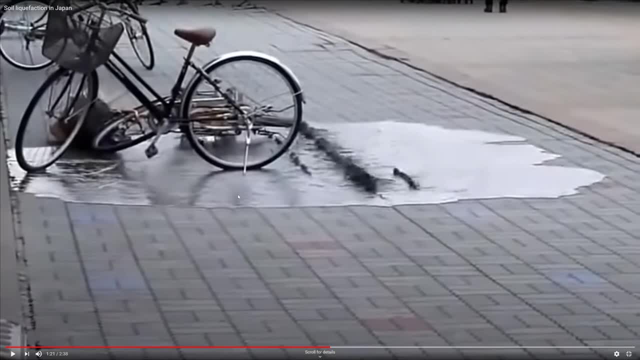 evidence of a sand boil. Okay, So you guys match the example of solid liquefaction in the lab, right? The situation is that we are working on solid liquefaction and we're able to find solid liquefaction in the lab, So the next thing that you have to do is make sure that the layer is strong enough to. 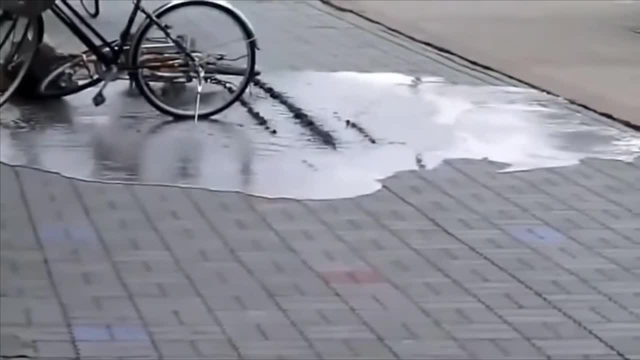 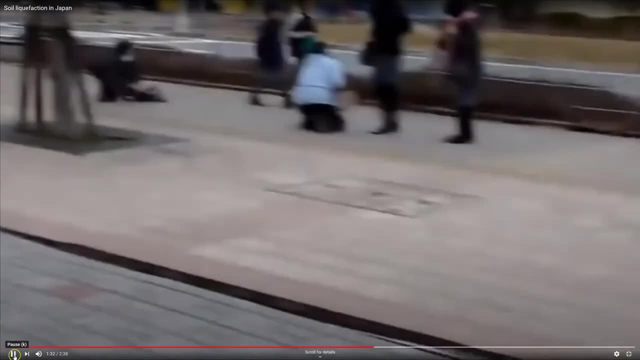 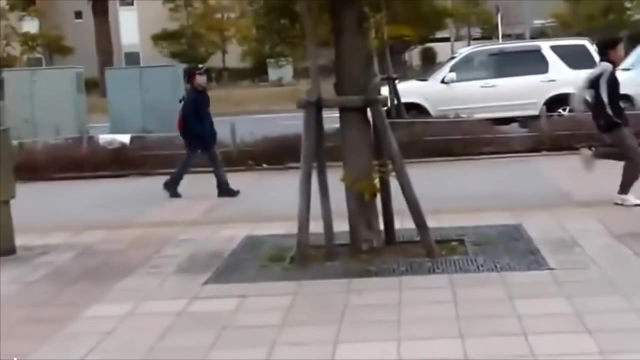 see the field. So we have. we have three layers of soil, like soil right. The first layer is not solid liquefaction, It's a sand, So it's very strong, very strong soil. The second layer is not solid liquefaction. 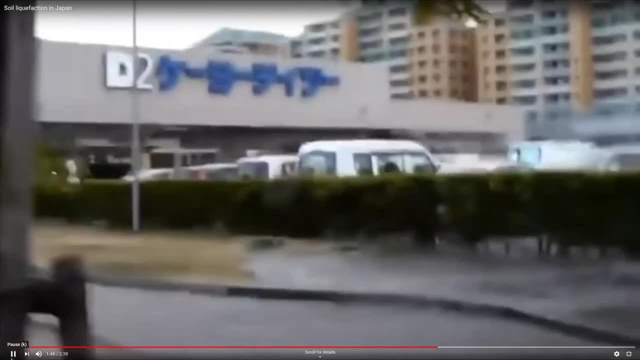 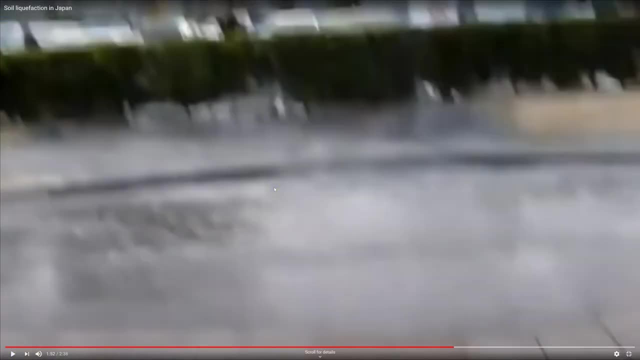 to come out because of the ground shaking. so with this, this huge amount of water comes out. what happens is that you reduce the devoid volumes of your soil stratum, then end up like you know you will: you create, you will lead to ground settlements. so, which is one of the the consequence of soil liquefaction, we 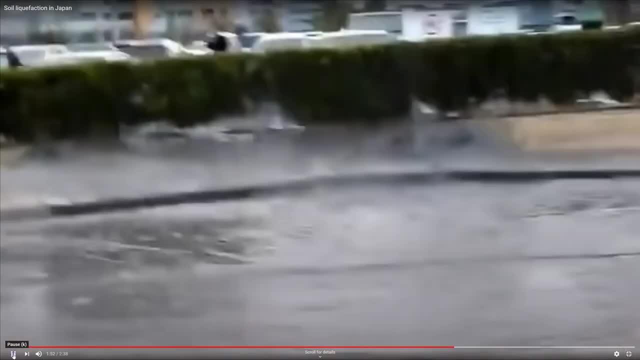 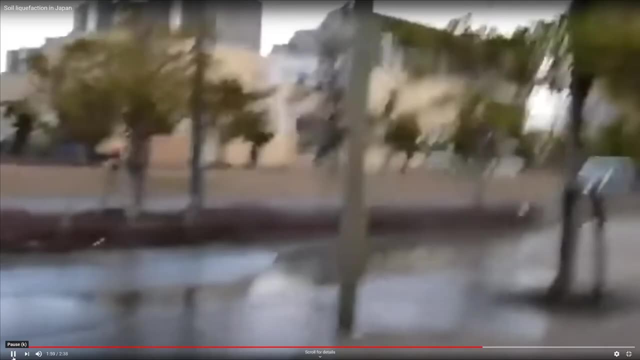 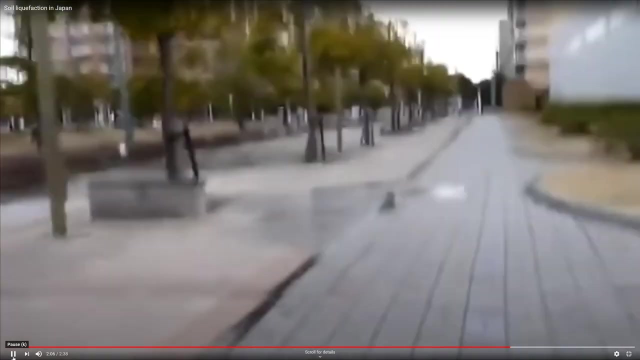 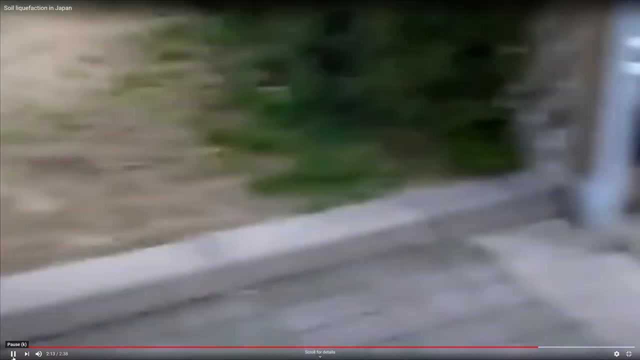 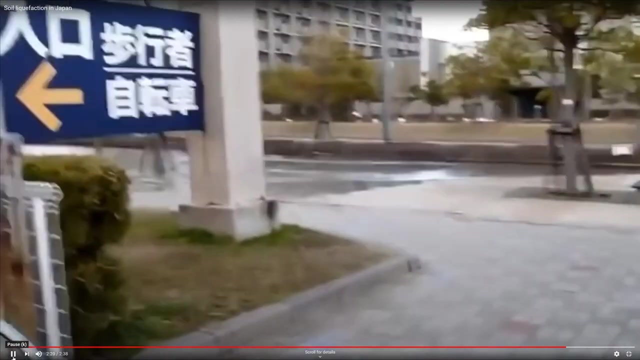 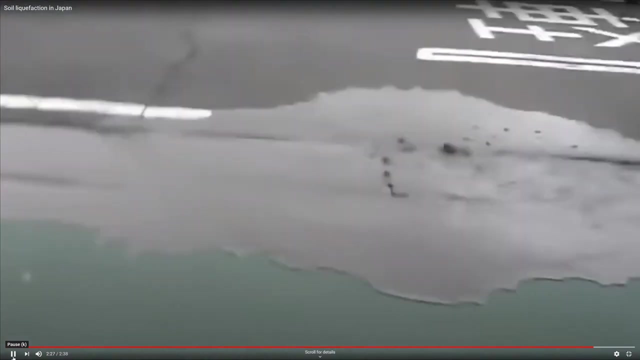 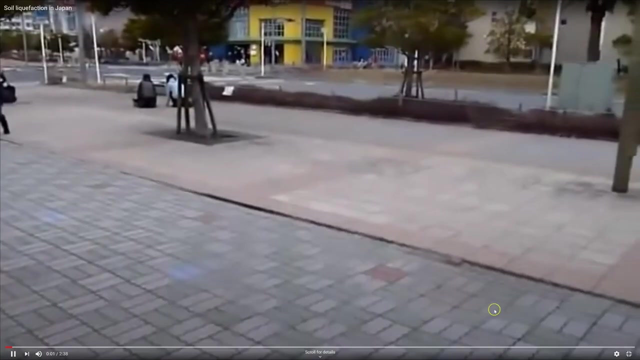 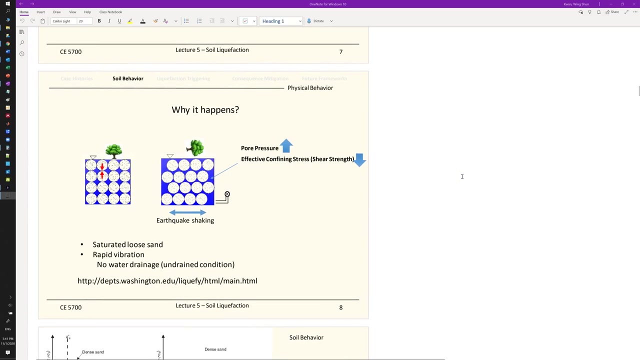 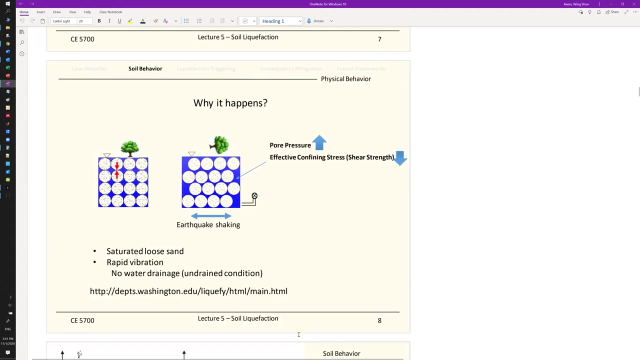 will cover in the later part of this lecture too. so more sand boiled water to come out, so okay. so why? why soil liquefaction happens. so let's take, um take a closer look on the soil behavior and um see what actually, like you know, causing uh the soil being liquefied. so, before uh earthquake happens, all the sand. 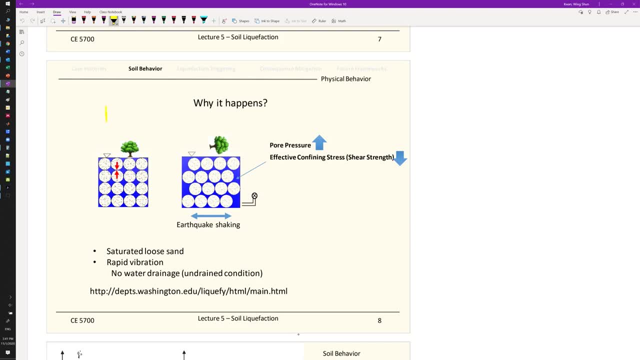 particle, uh particles. so this is like the uh before before earthquake. So all the sand particles. they are kind of like during the at-rest conditions. The sand particles are packing, kind of like as a structure, All the sand particles under the vertical effective stress and horizontal stress which provide like the confining to push the sand particles contact with each other. 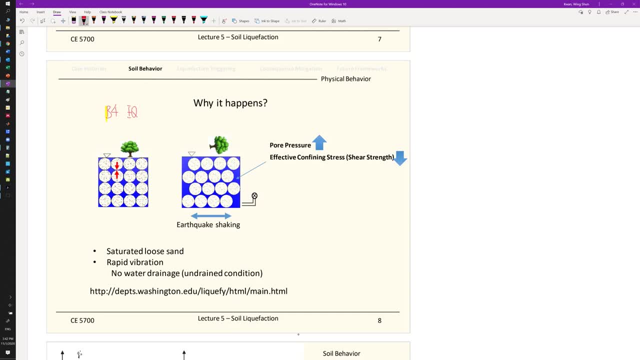 And for sand, the majority strength of sand come from the frictions. So as long as, like the sand, are under pressure contact with each other, so that's, the whole soil structure is intact. But what happens is when earthquake happens. so when you have about 10 to 20 seconds of shaking, just like the ground motions that I just showed you. 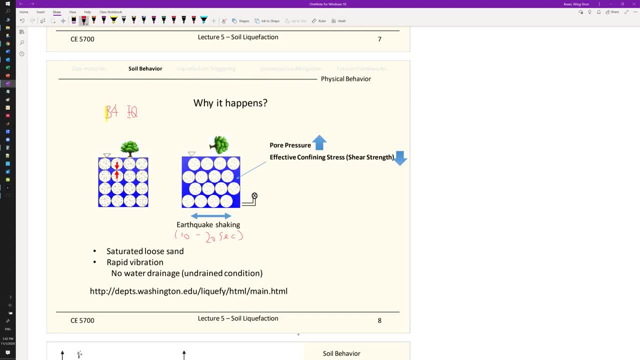 that you guys have been playing with since lecture number two. So when earthquake happens, the sand particles. so what happened here is the sand particles. they wants to get into a denser configurations, So try to get into a denser configurations, But what happened is that the water is trying to prevent this. 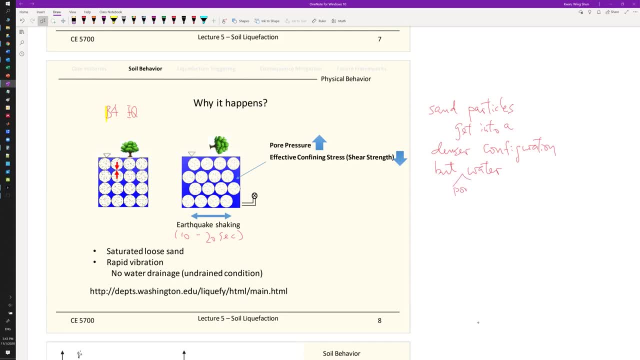 Well, the poor water. so the water trap between the sand grain right there, the poor water prevents it. So therefore, there's you actually just like a no volume change, just because it is under the undrained conditions. It is undrained here, So when the shaking happens, there's no time for the poor water to come out. So we, you know, just like you know, we wash the. 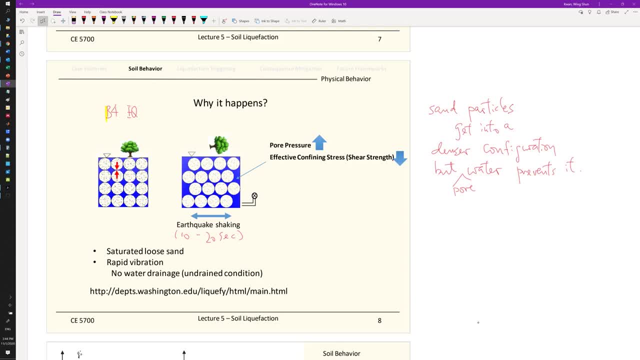 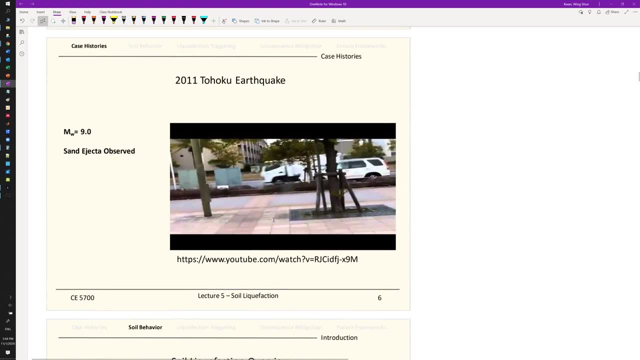 to oku. So you realize, by when the shaking start you don't see the water come out because the rehy perto de la momente anterior, abyan, it's just like a liquid fractions in progress. But it will be at later part of the earthquake or after earthquake being finished. So that's the time. so you hear, you have about like. 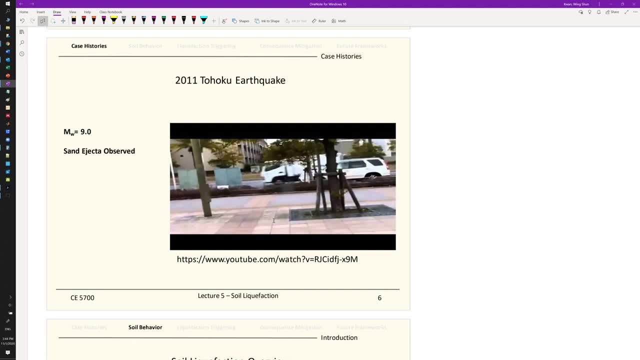 ten to depends on the financial five seconds ofiforn continues to come out depends on the following time. So you will have about, like you know, 10 to depends on be fine contents. So you have M. Three other things like: oh yeah, it's really very different. 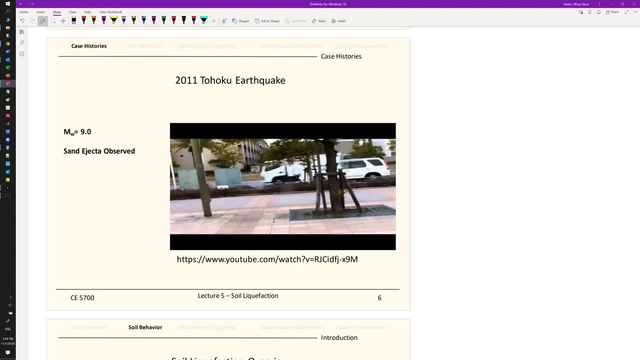 Yes, I hope I have the first, Yeahriobra one has only twocję movement than m? e. and then we have the second, because Port Imperial, in addition to the, have, like you know, uh, uh, like 50 or 60 seconds right there, uh, what happened? is this under the 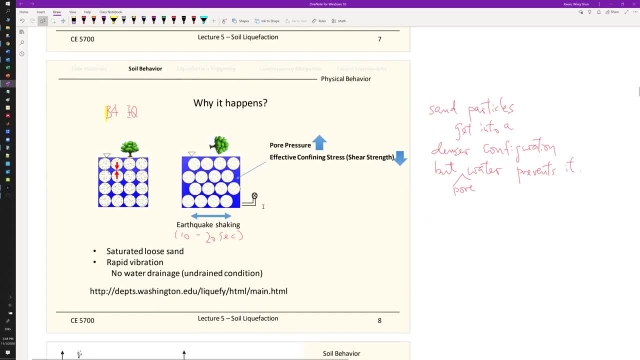 undrained conditions, just because there's still no time, uh for the portals to to to come out, uh, from the soil areas. then what happened is, uh, this give us the undrained conditions, so this is undrained it, so no time for water to escape. 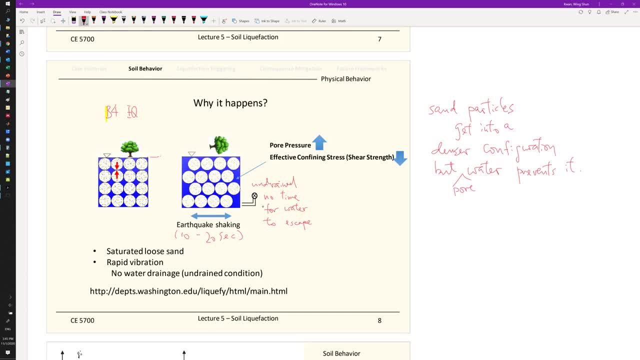 and like: even though the volume is not changing. so during that process, you will see, like you know, the volume is not changing, there's no volume change, there's no settlement, uh, but what happened is like the product trying to shake. so, at the micro scale, what we hear is: you start to lose. 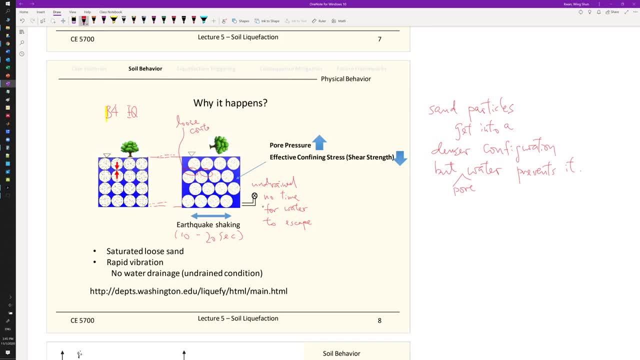 contact between this all the same particles. so you've that. if that happens, if that happens, so this it will be- becomes like the pore: pressure will be increased because you know what happened. is this the sand? you know the water, water comes out, but you just you know you cannot, so you create like our. 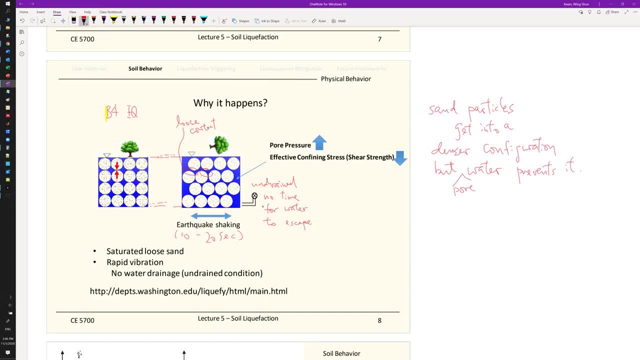 pore pressure and also we started to lose contact. it is between the sand particles then end up like the effective confining, stress would decrease and this can explain, so this part, why the you are the string. we lost all the source strength and this can be explained by the decrease. you do refer to the 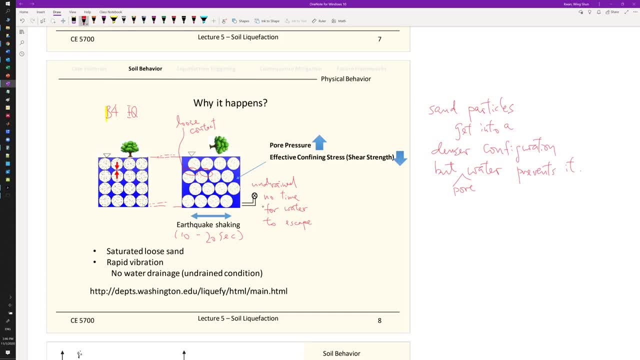 effective confining stress due to the increase of the porous. sure, this can be explained by the uh, the psychic effective stress uh theory. so which is the effective stress equals the total stress minus pore pressure. so now the pore pressure go up because of the shaking and because of the generated, generated excess pore pressure and the vertical effective stress will. 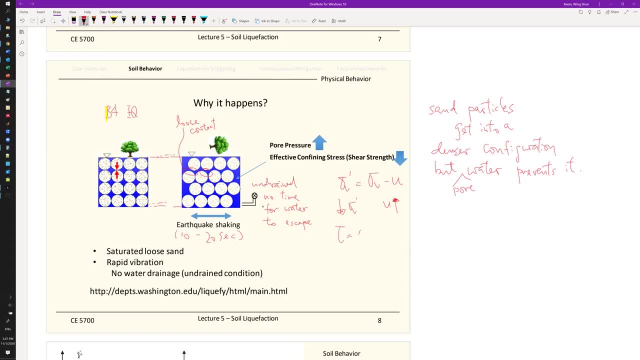 go down and we know that the shear strength of soils is equals to the vertical effective stress times, the tangents of the uh fee plying. so the friction is a key uh. but if you're losing all the uh vertical effective stress, then your shear strength almost go to zero. so when uh, your 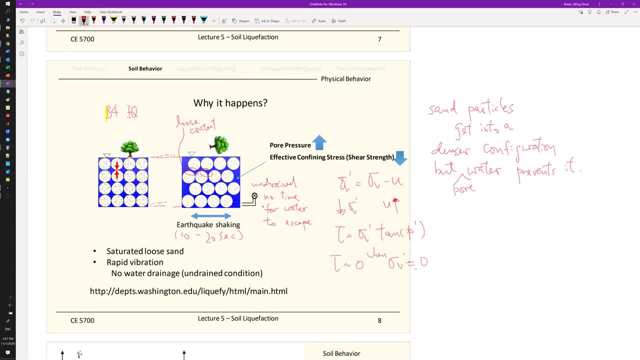 vertical is effective stress is about to go to zero. so this could happen when, like you know, uh, your generate generated excess pore pressure is about equals to your vertical effective stress, or the actually the total stress. so if the excess publisher generated is almost equals to the total, 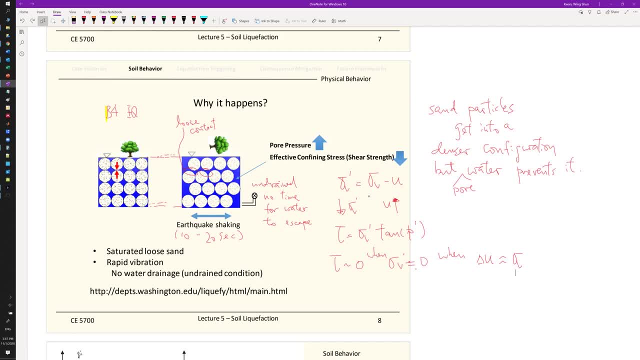 stress, then you lost all the soil strength and that is the full type of, uh, uh, solid core fractions to be happening. so that'd be quite, quite dangerous, because now, uh, pretty much like you know, uh, the whole sand area will, will be gone. so is that what? that's why you call it liquid fractions. 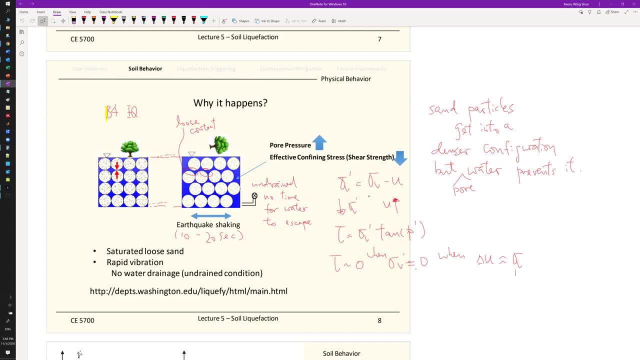 because now the salt becomes just like liquid. so it's very dangerous, uh, when uh there's, you know, there's no strength at all. uh, or when, you know, when solid quifactions get to that point. so in order for this like a solid quifactions to be happens, uh, it only happens on uh saturated loose. 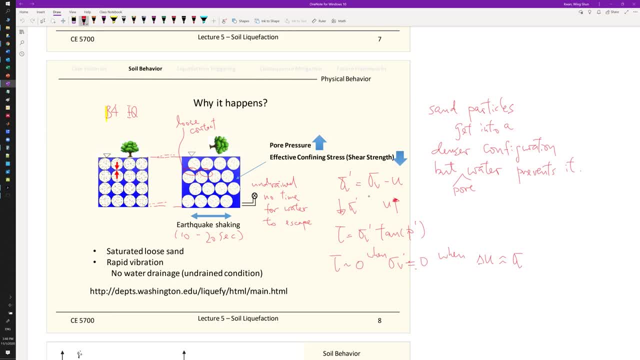 so when you have a loose set uh configurations, uh, with water being there, uh, you know, submerged by the water table, uh, that's where we were about our solid quifactions. so when we say loose is like, uh, less than 40 percent of relative density, but that doesn't mean like the densified, the dense, uh, sand. 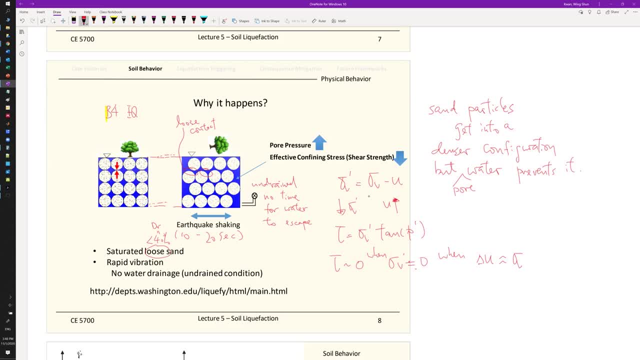 won't liquefy actually. uh, you know, when you get a 60 percent of density, we also quite worry about and uh, but when you have very dense sand layers, this may not be as dangerous as a loose one, but you, you will liquefy it. here. we can observe that in the laboratory data. uh, which is a little bit. 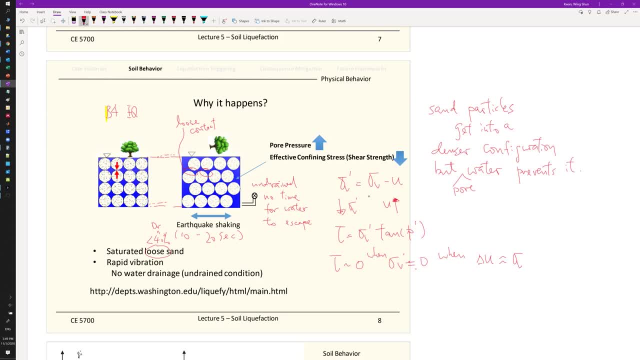 different of like uh, stress path, uh, you know we talk about stress part 3566, uh, but you will, you will also happen from densified soils, but it may not be the full type, the full type of like a uh, a failure. you, you will have cyclic mobility. so we talk about what is psychic mobility. 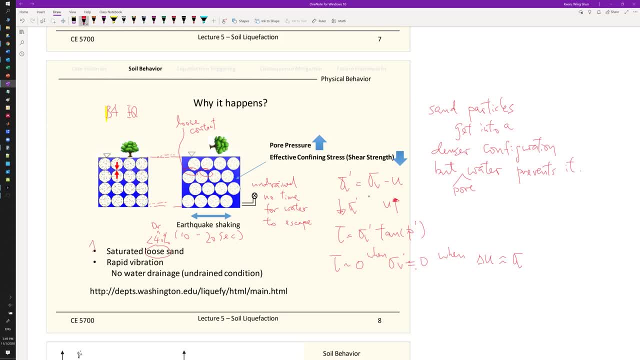 so you need to have two conditions: first, you have uh saturated sand here. seconds, you have rapid uh vibrations. so that's, if you fulfill those conditions, uh, we're about solid quifactions. so that's why we're about this in california, uh, because uh rapid vibrations. yes, it's kind of like you know, we know it's always there, which? 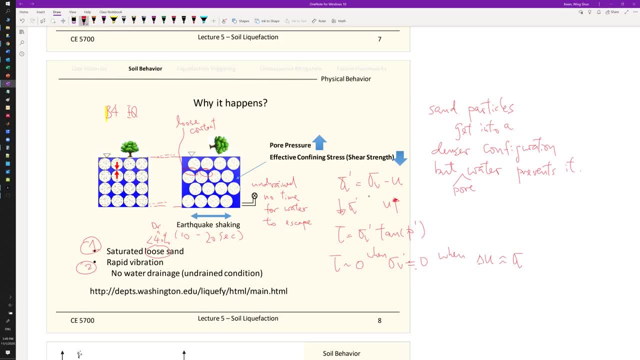 means the earthquake loading. uh, it's a potentials you will have that uh. other thing: like you know, new industry- they have the blasting loading. so when you do the blasting uh the as the mining site, uh, you worry about solid refractions on the site here. so you need to make sure everything is. 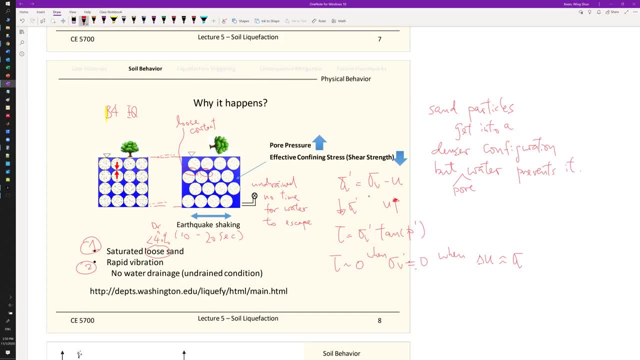 safe uh. other like a y vision loading could be uh like a sea wave floating if you uh design for uh the drill path внут�� offshore, those like uh c wave flow, those wave floating back-and-forth, those serve as like cyclic loadings too. 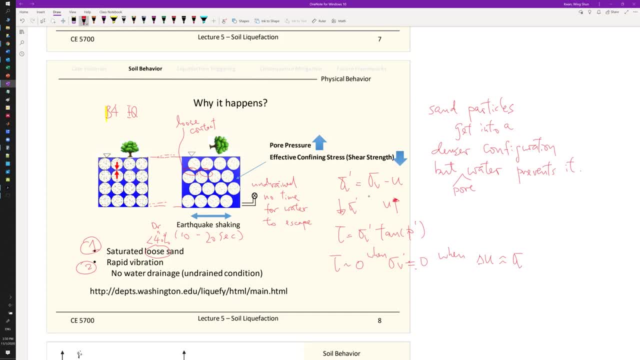 And for more information about the background, sort of like a fractions. This website helps this out. It's kind of like a 20 years old website, But is the works is by a Stephen Kramer to offer the textbook, Which is, which is very nice. So if you want more information, so feel free to go to. 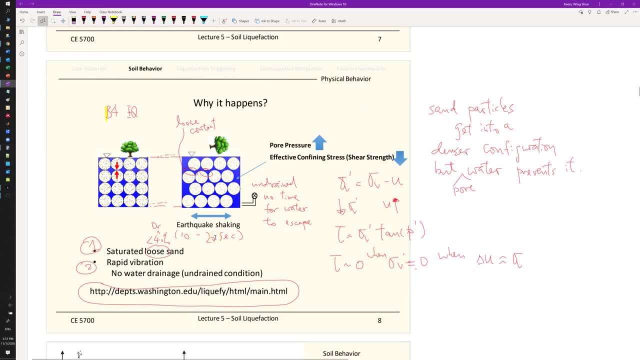 This website is a little more and, with your textbook, sort of saw a Stephen Kramer, Almost a saw Kramer, Stephen Kramer, He is. His work, his entire career is based on Sort of confractions, signing a PhD up to you know, He just retired and he got elected to NAE, which is the National Academia of Engineers. 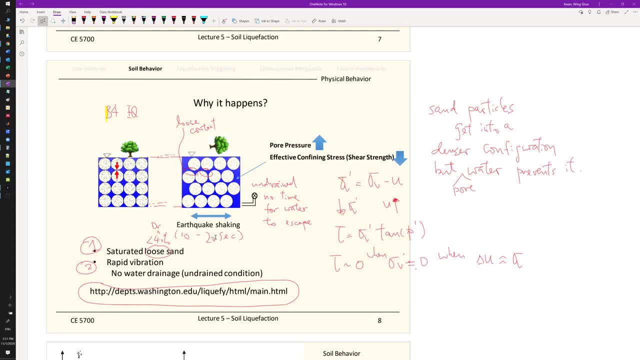 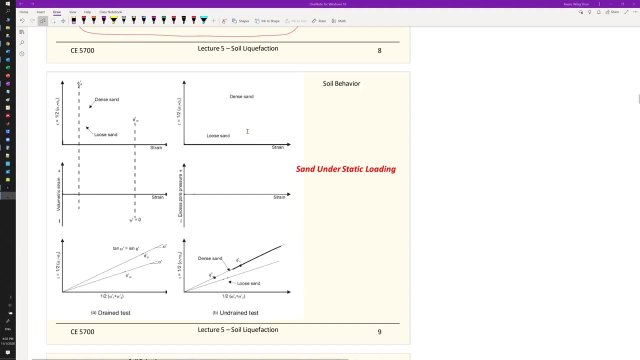 The highest at honor or the highest, most prestigious award you can get as a as an engineer, And his main contribution is in this topic- sort of confractions- Okay, Sam, behave here. so I Quick review on what we have learned on some mechanics. so for sand, how would the 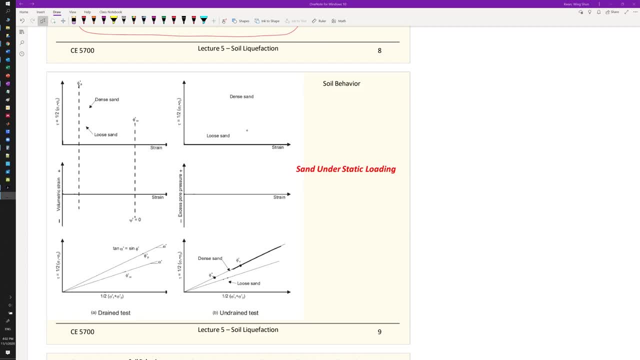 Sand elements behave when you're subject to Represented by stress-strain curve. so if you have A very dense sand, so this is kind of like the stress-strain behavior, So you have the peak Kind of like the peak friction angle, And then you will go to the critical state and then you're pretty much you have the 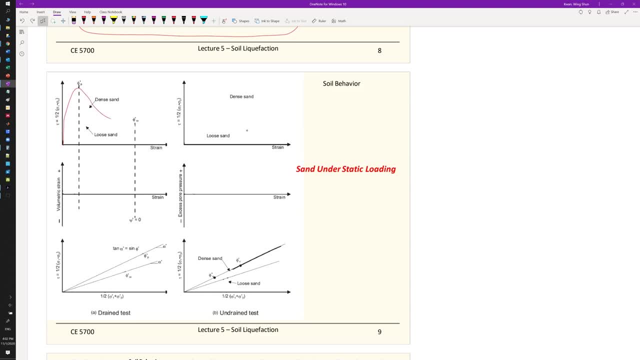 the constant of volume friction angle. So here the C sub V stands for the constant volume. Now the P here is the peak, Now the P here is the peak. So peak friction angle and constant volume Friction angle. and if you have loose sand Then you get a stress-strain curve like pretty much only defined the constant volumes like a friction angle. 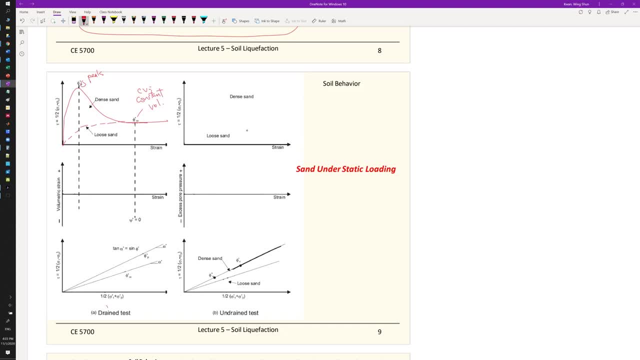 So if we, if we consider this under the drain behavior- So if you're wanting a CD test like kind of like the tracks you test consolidated during test, You are, you're not matching the pore pressure, but you like let the drain gauge open. so make sure you're loading is slow enough for the. 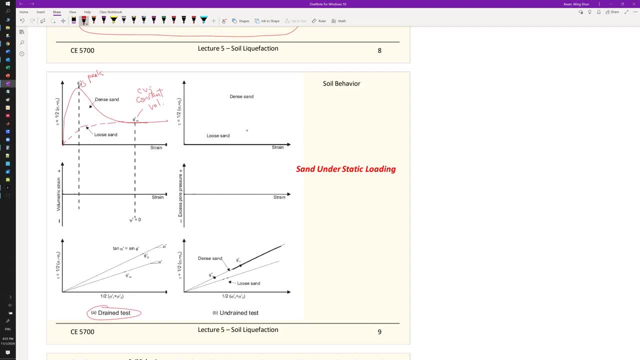 Water to dissipate it, excess water to be dissipated with, though, like you know, building up off excess pore pressure. then, like you were for the, the dense soils, you will have the Dilative respond. So this is the dense soils, and for loose soil, pretty much like you will keep. 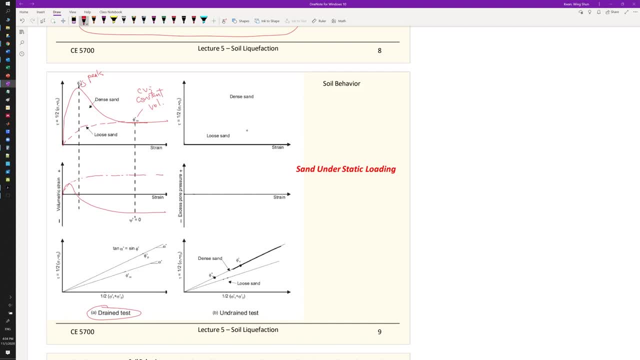 Loosing up. so What? so? this is geotech convention. right when this is positive, means compressions. So if this is your sand samples, sand tractive samples, for example, If this is like a shortening, Then this is a positive, But like if it is like a extending. 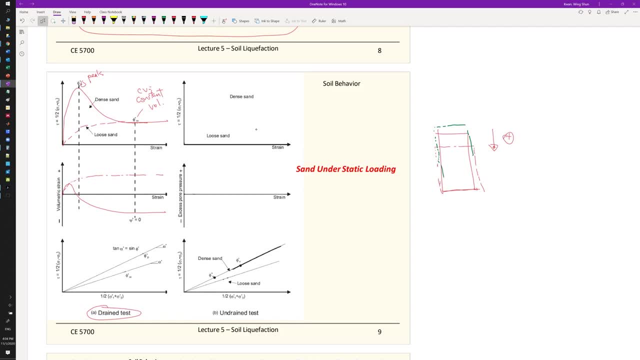 Like dilating. if you have dilative respond, Then this is a negative. so when you have again, you know this is This? all mechanics. we talked about five, six, six up. when you have a dense soils, they try to Sheet against each other, So the the soil particles try to roll over each other. So that's why you extend the volumes. 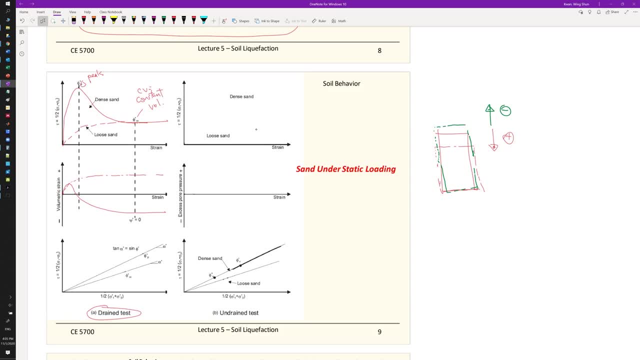 But if you have a loose sand samples, They will try to get to a denser configurations so that will give you the, the positive volumetric string change. So that's why, like you know, the the tendency of try to Reduce the volumes. This is very dangerous for solid confections, for the, especially for the loose soil. 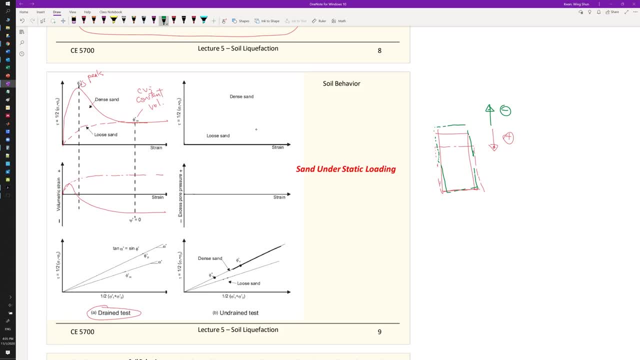 And when you have a stress path, This will kind of like a go straight here now for both dense and loose soils, because everything is like drained it. So that is kind of like the stress path and you will be heating both like our constant volume, our critical state envelope. 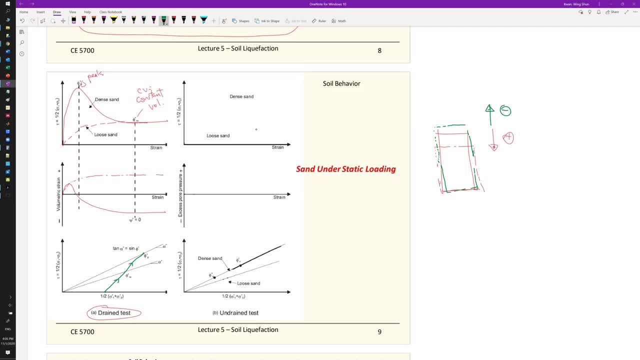 So you know the slope here which is the friction angle. So it represented critical state, CSO aligned. so critical state, aligned right there. So similarly. so this is the drain test for undrained behavior. So you are measuring. So again, this is the total stress base for the 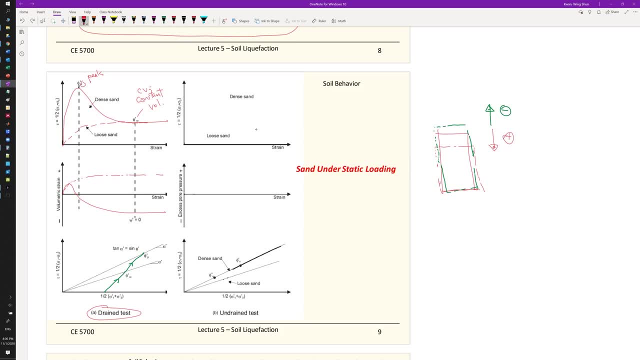 undrained behavior. so pretty much this capture both, Because there's a buildup or excess pore pressure. So your stress strain curve now we flag both Pore pressure and excess pore pressure and also the Effective stress. so that's why I, like this curve will keep going up, because you know you're considering the generated excess pore pressure and 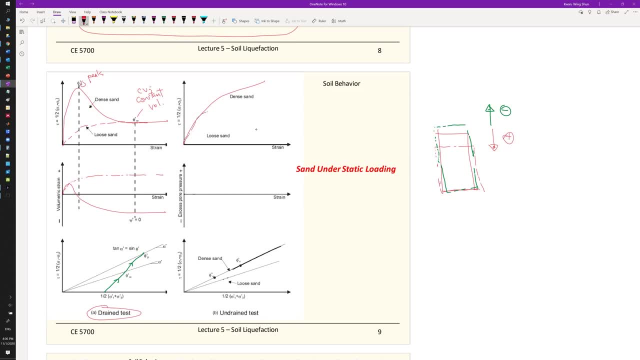 For the loose Soils. it's kind of like the same too, but you will kind of like a peak out. So this is the loose soils and this is a dense soil for undrained, undrained test, For undrained test, you know. 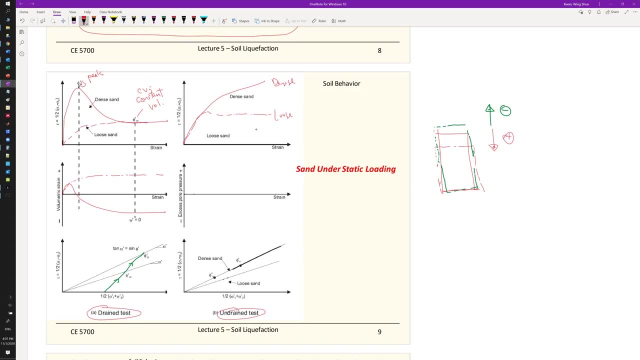 We are not measuring the volumetric change because the volumetric change will stay the same same, as, like the drain test, the excess pore pressure is zero and. But when you read your undrained test, the volumetric change will be zero, but we're through with generating excess pore pressure. 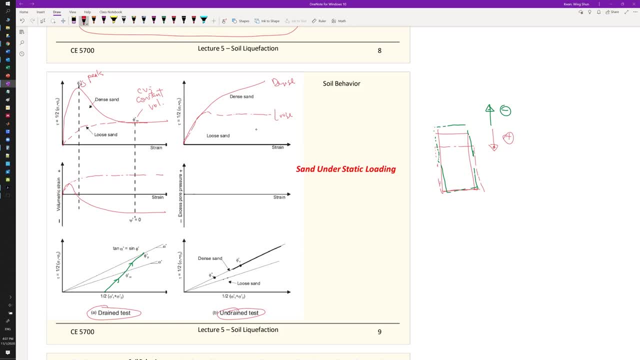 So that's why I like the liquid fractions. when it happens, This is an undrained behavior. There's like a no volume change but generating excess pore pressure. and for loose sand, you will be generating the excess pore pressure, And for the dense sand, first You will generate a little bit of excess pore pressure and then you will get a negative for excess pore pressure, You keep dilating. 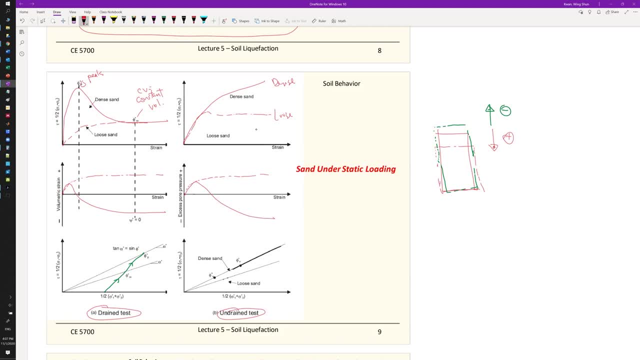 Like that And for the stress path for the for the loose soils, You first, like you were generating the, the excess pore pressure, so finally you will, goes to your critical stay line and for the Loose- uh, I'm sorry for the dense soils, the stress path will go this way. 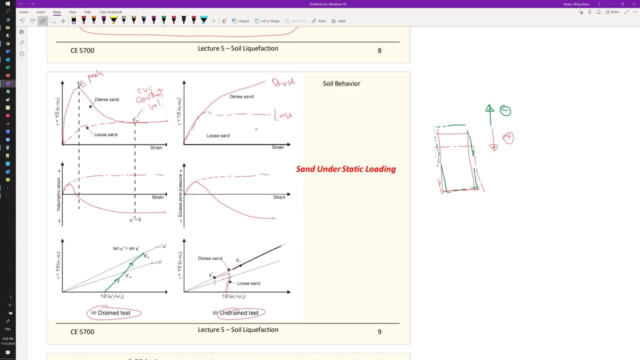 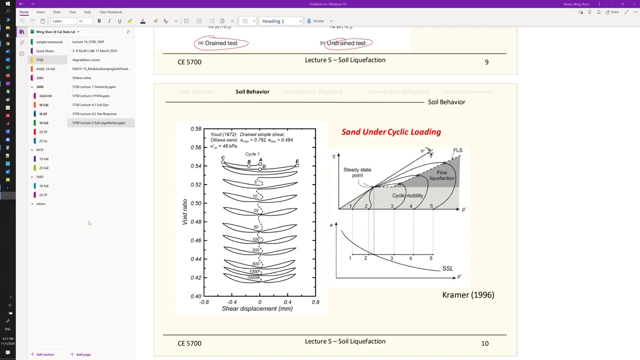 So eventually. so both of them will still heating the up the critical stay line. So this is This is the loose one And this is the dense one. Okay, so this graph here. So how the cyclic loading work. So first, like on the left, it shows you. 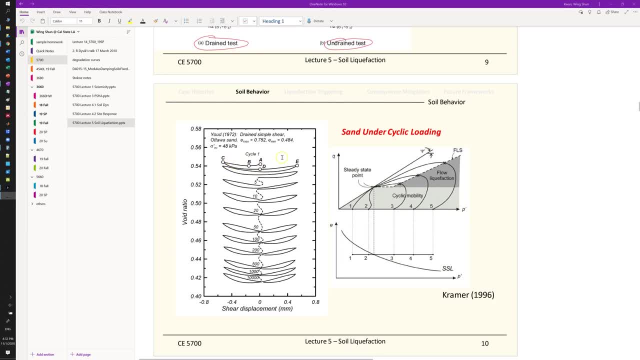 Under drain loading. So if you have us back and forth our cyclic Displacements imposed to the soil samples, You will see that, like you know from very beginning, you have your first loading cycles to the end. so you know this subject subjected to a very small loading, but you go to 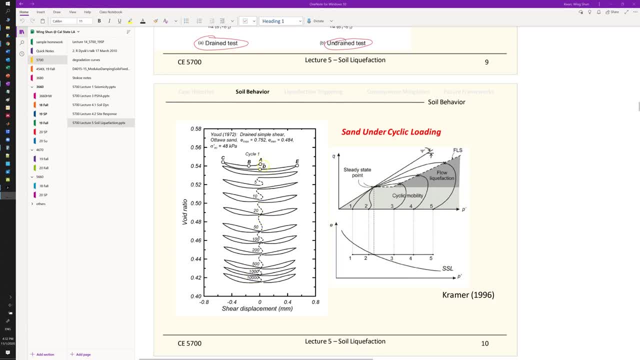 a thousand Loading cycles. So at the first loading Go back and forth like dairy, So you randomly keep Loading your soil samples, You will reduce the avoid ratio, So the whole thing is getting Densified. so this is like a drain loading. you know. you could happens on a dry sand or like you know. 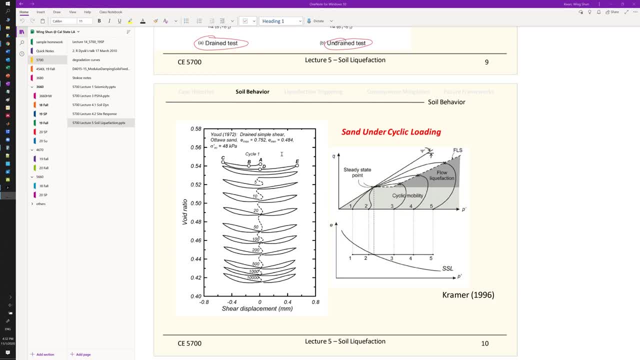 saturated, saturated sand that allow drinkage to happen. so this is a proof that in fact There's like a volume reductions when the psychic loading happens and this on the right hand side shows you like you know the stress path and you further explain the concept of full liquefaction and psychic and psychic mobility. so this one psychic 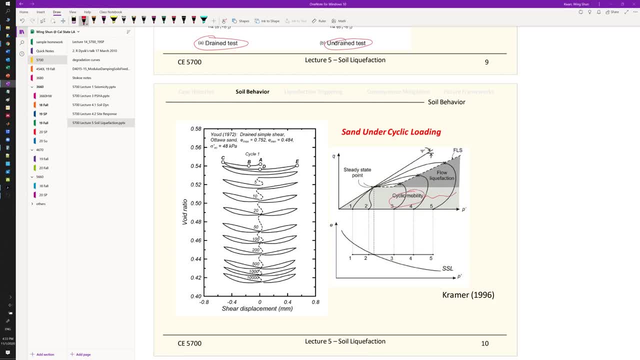 mobility when you are here so you only like limited excess pore pressure is generating. so on that part pretty much like you know. you know better be more like at the beginning of loading when you ever dance all zambos, so only limited like reductions of salt strength. but when you get to this 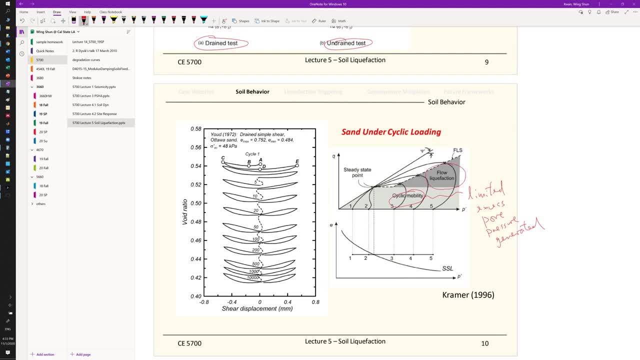 part. so just out like this stress path, you know, think about figures, you know how the soils, how the stress like, go from one point to uh, to the steady state, and when you get to the later part, here the full liquid fractions. this is very dangerous because uh. 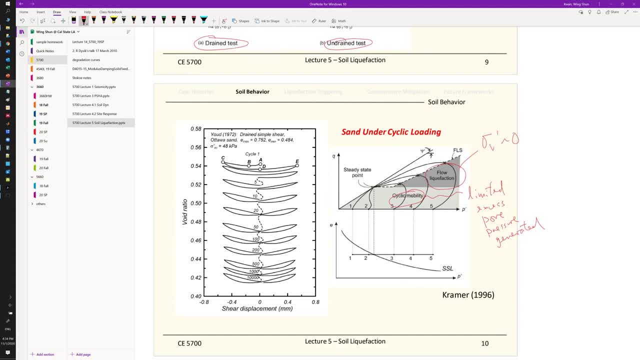 at that part your vertical effective stress is start close to zero. so, pretty much like you know, you almost get to the point of losing all the source strength. so this is, this is very dangerous. so that's why, like a loose sand, uh is dangerous because, uh, you will easily go to liquid fractions. 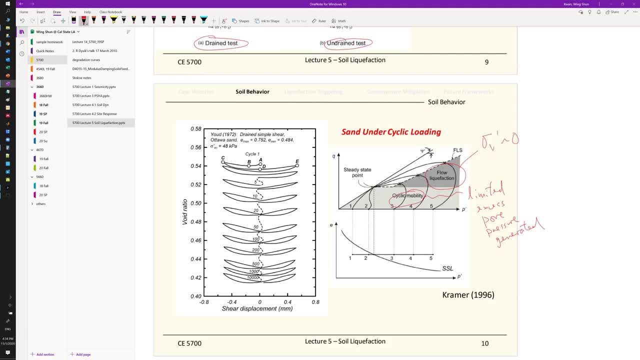 uh the full liquid fractions, uh uh stress path. um, but versus the uh dense ends, you know, at the beginning. uh, you, you may uh end up at the second mobility without going to the? uh the full liquid fractions, uh route over there, and i got this line here also: uh define the aesthetic status state. 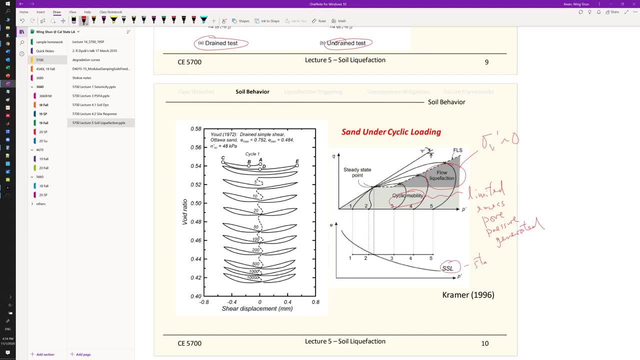 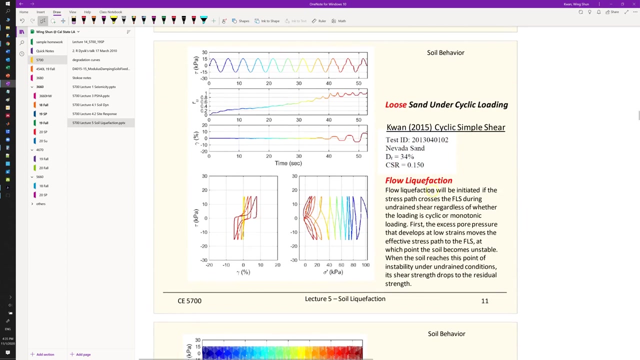 line. so this is the statics, uh, the static, steady, oops. all right, right there. so here this also choose some uh experimental data from psychic, simple shear cast. so we have a input like a stress, um stress history there, which is the harmonic motions, uh with, uh about. 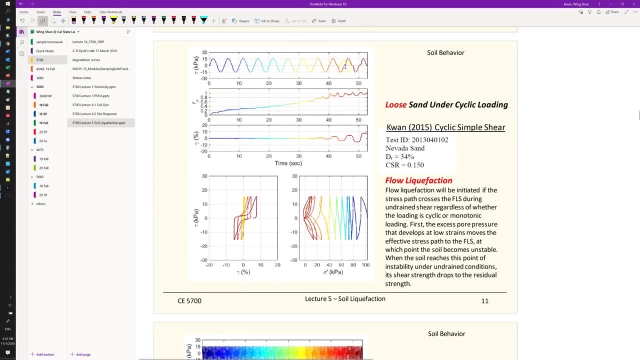 10 cycles. right there and you see the uh. The color code helps you to see the generations of excess pore pressure, shear strength. So this, the second row here, is the excess pore pressure. So L sub u here this is the excess pore pressure ratio. 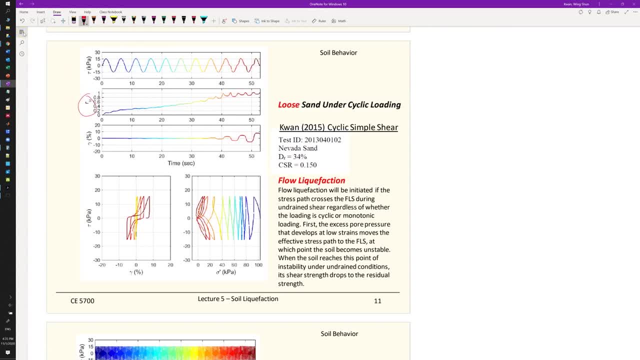 So L sub u is the excess pore pressure ratios And L sub u is defined by the generated excess pore pressure developed by the initial vertical stress. So, before the earthquake happens, what is the initial vertical stress? So let's go to the denominator. 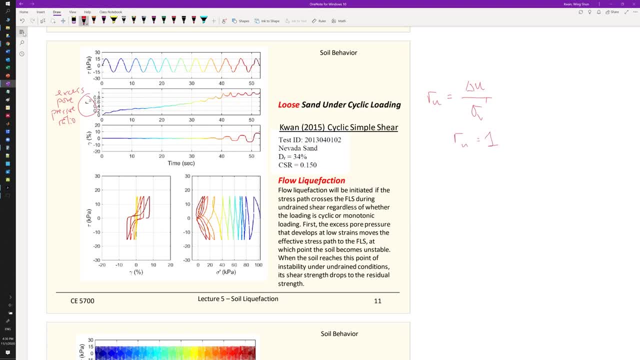 And so that's by when R? u equals 1.. You lost all the sources, So that's just the follicle fractions Or the failure. So when R? u equals 1, then that's where, like the moment, we lost all the source strength. 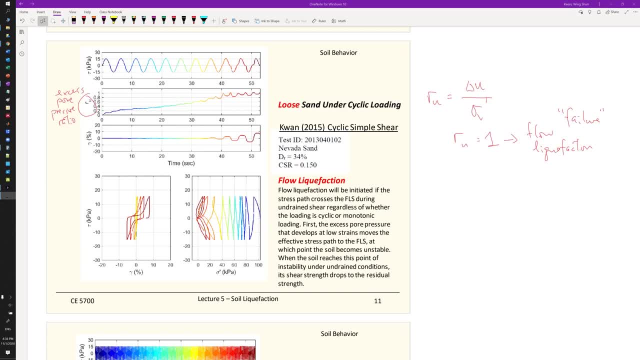 because the generated excess pore pressure is as large as the total vertical stress. So when R? u equals 1, then there will be like for sure it's like a failure, Failure, Normal source strength And again, like you know, this is the input shear stress. 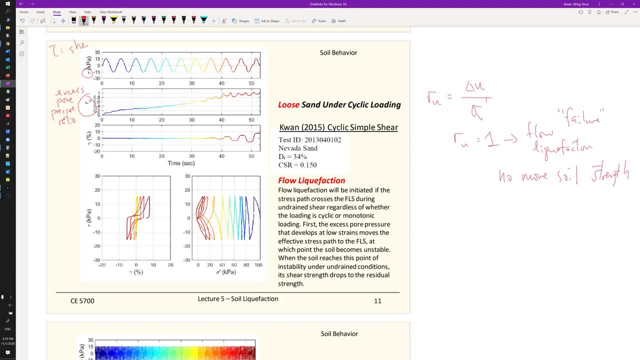 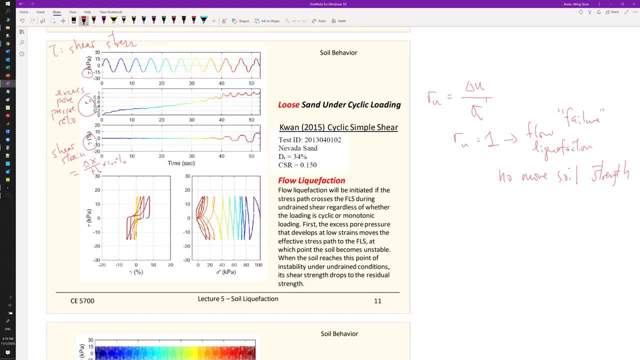 so when you fell the Minnesota sample fell, there's a lot of like a fairly deformations. so you know it's telling me meeting like the ground surface where you have expecting a lot of like this placements, and this is another graph. so I need a stress string pot. so we talked about this a little bit in the soil. 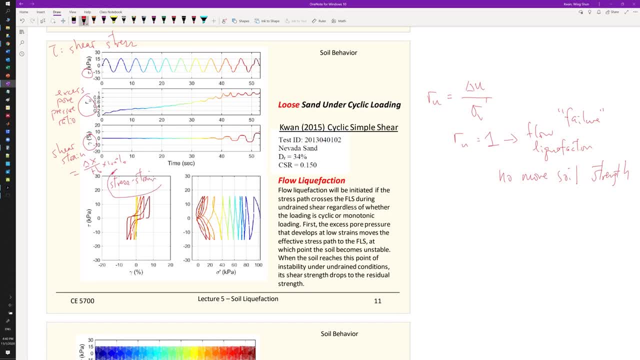 dynamic properties like a lecture. so this is the stress ring plot. so the blue one is the initial circles, which is like over a tiny tiny at the beginning. when you close the failure, you generate a lot of like outer spacements. so it this is the stress ring loops. again, the areas of the loops represent the dissipated